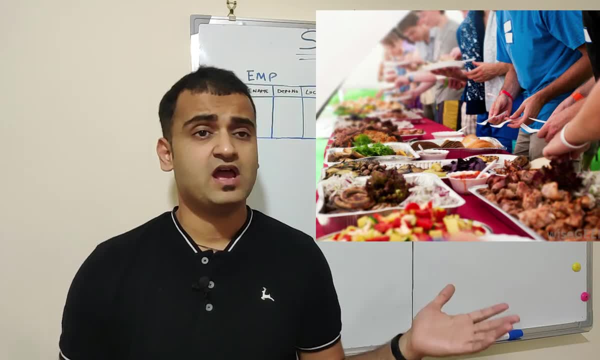 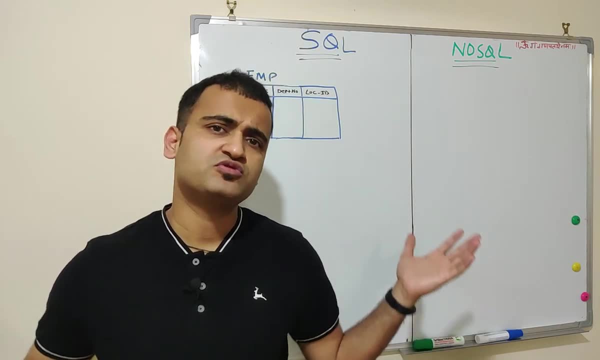 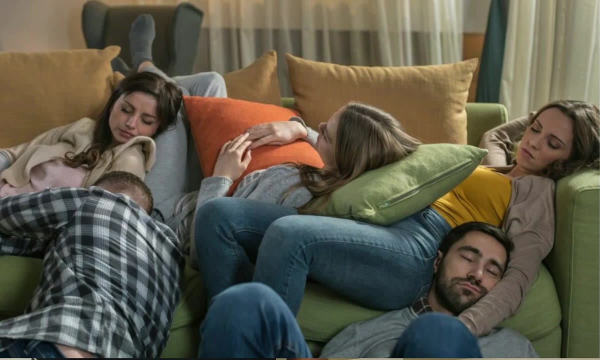 And you will make food arrangements very flexible which anyone can have. You can have accommodations, maybe open your whole house. if anyone wants to stay over, They can stay. they can use the stairs, they can use your sofa, your pool, Wherever they want to. 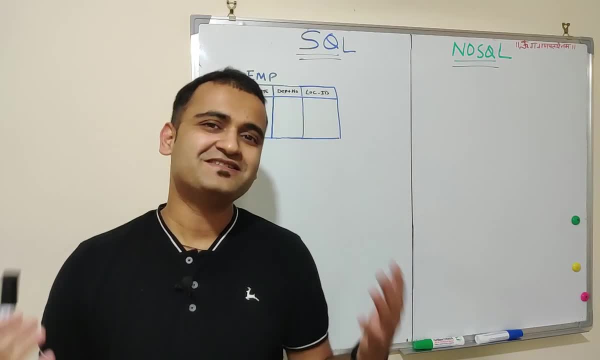 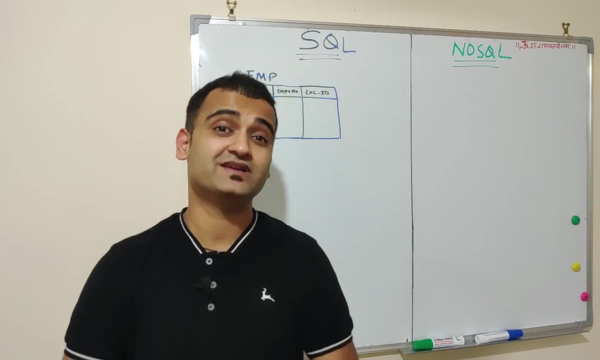 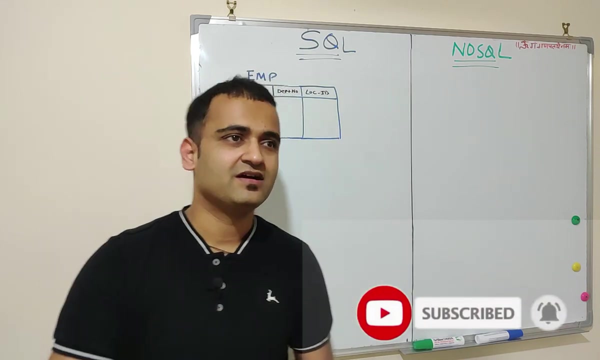 So it's an open house party which you have kept this time. So, in a similar way, instance 1, where you had a fixed set of guests coming in and you had all the plans, likewise Was a very, very, very clear case of you trying to feed data into your traditional SQL database. 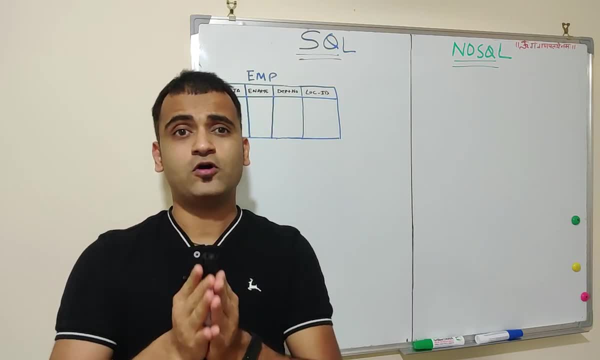 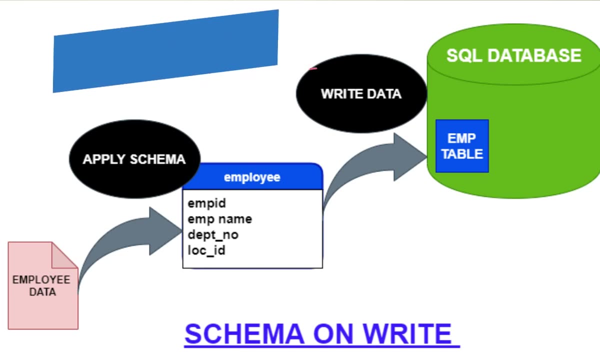 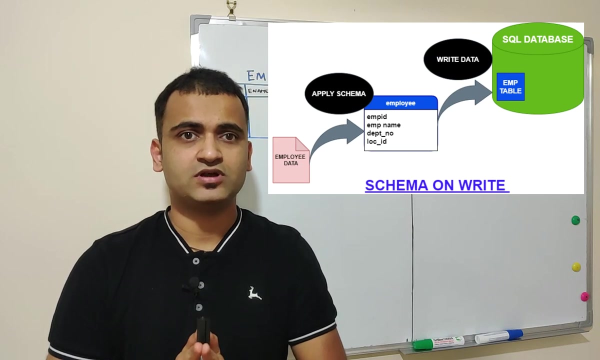 So in a traditional SQL database, you follow schema on write philosophy. What does that mean? What is a schema? Schema is a set template which is predefined and you expect the data which is trying to enter this particular SQL database to be precisely in that same format. 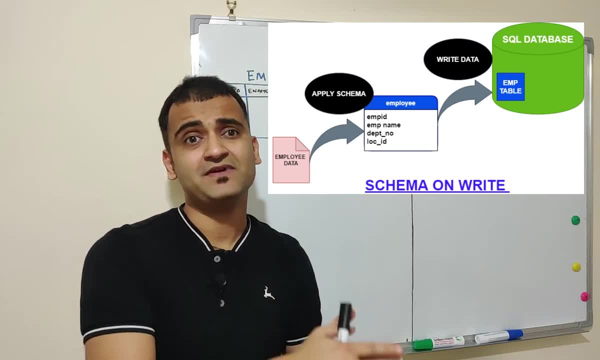 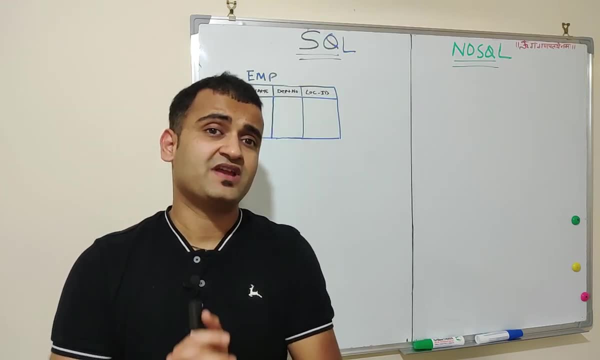 You have to make sure that there is consistency in the way the data is coming. If there are any last minute changes in the data, in the format, then traditional SQL databases tend to struggle a bit. But a NoSQL database runs on philosophy of schema. on write. 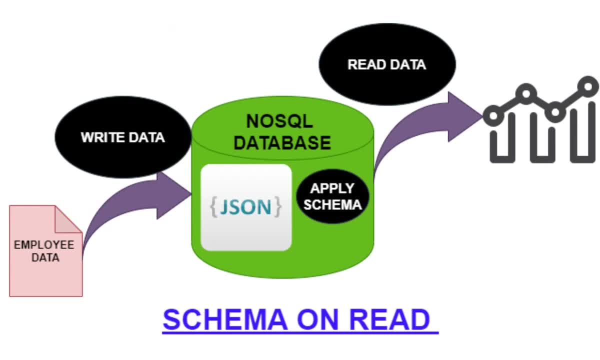 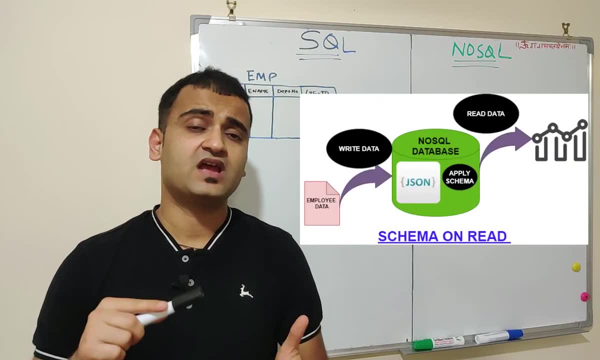 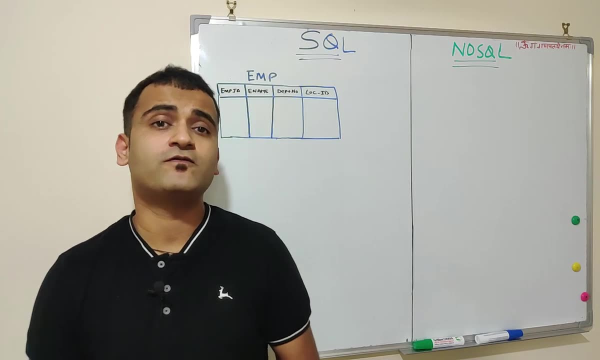 Which means that a NoSQL database is ready to accept any kind of data while it is entering into the system. It can be structured data, it can be unstructured data or it can be semi-structured data. So now, as we have a basic understanding of what is a SQL database and what is a NoSQL database, 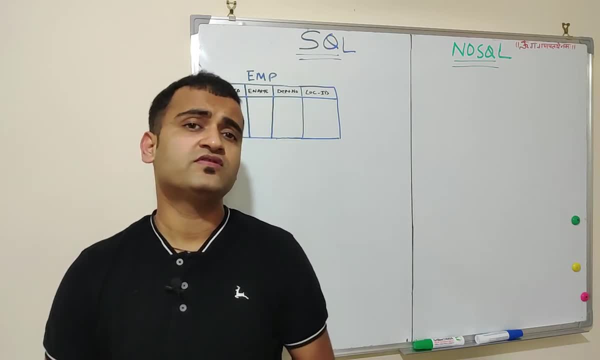 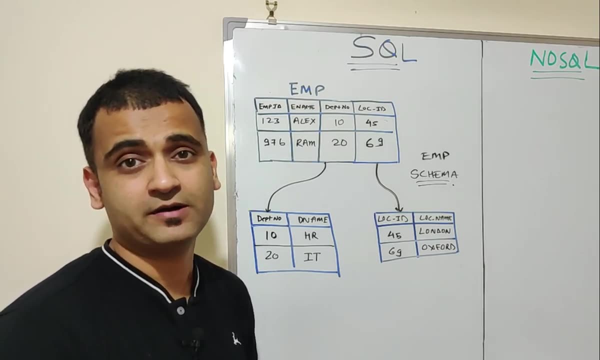 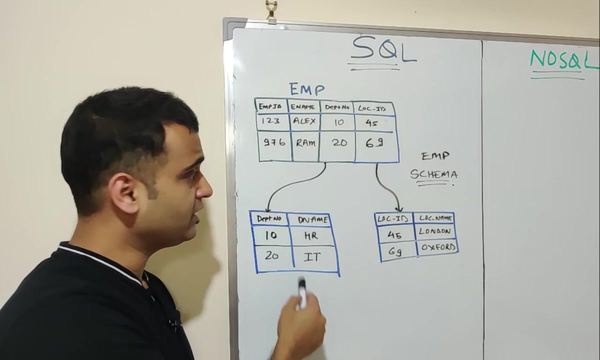 Let's dig deep into the concepts with our famous employee table example. So, as you can see, this is a traditional SQL database. This is an employee table containing all the details of an employee, And then you have subsequent data stored in department and the location table. 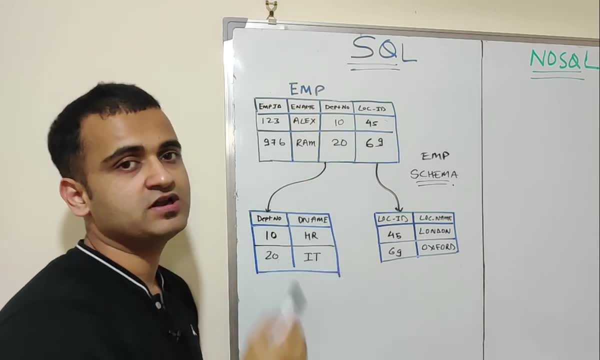 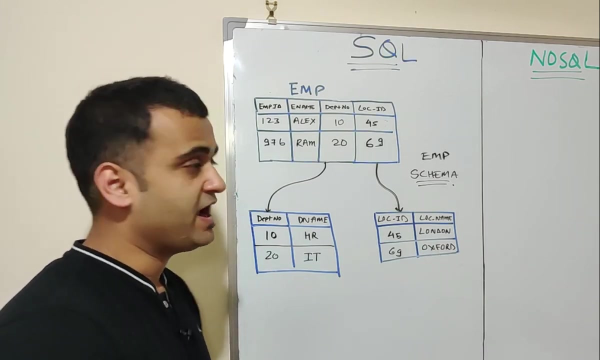 And you have the keys, primary key, foreign key, relationship between these tables. So if you want to understand that which employee works in HR department and stays in London, Then you have to run a query, And you have to run a query and join the data based on these keys. 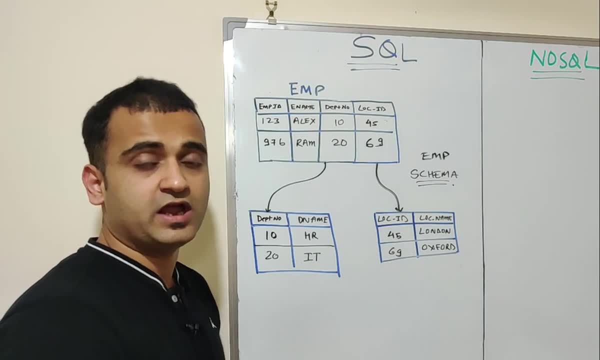 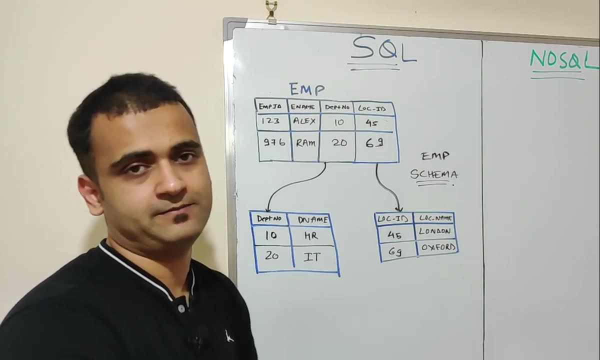 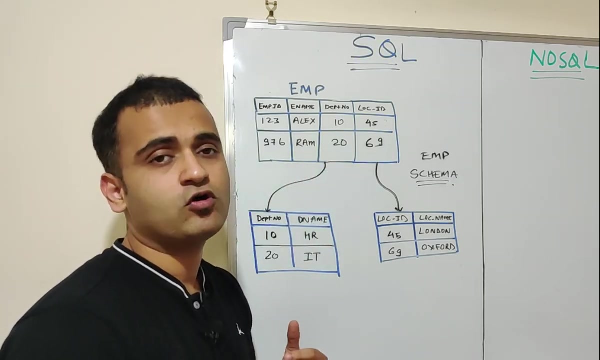 Now this is a fixed format in which the data, while coming into this kind of a database, would expect the data to be in. But consider a scenario that all of a sudden in the employee table there is a structural change, And what is that change? 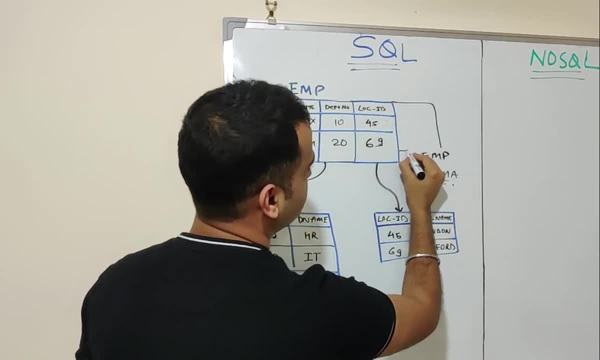 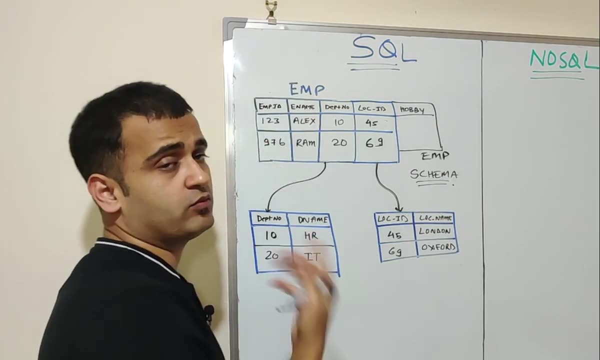 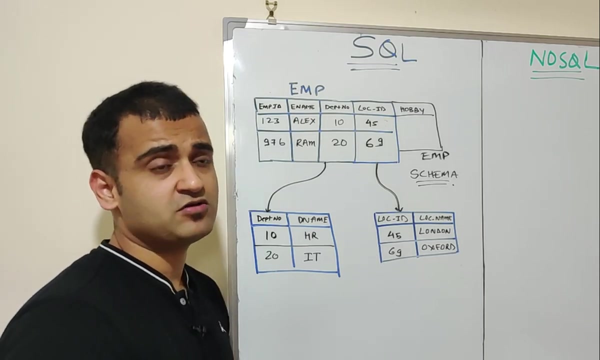 You have an additional column getting added, And this particular additional column is called as Hobby, And this hobby could vary from one employee to another, First of all. Secondly, there could be instances where an employee does not want to enter this data into the system. 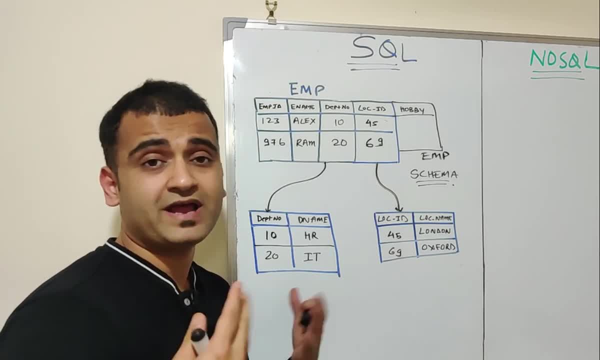 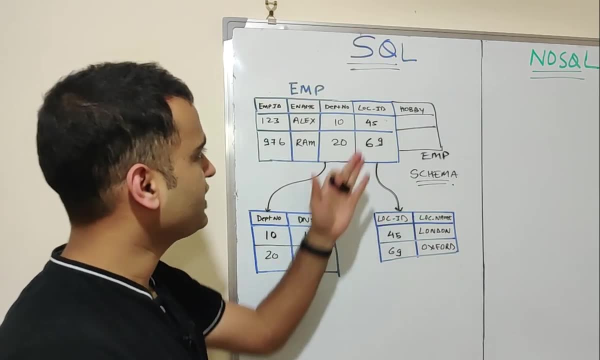 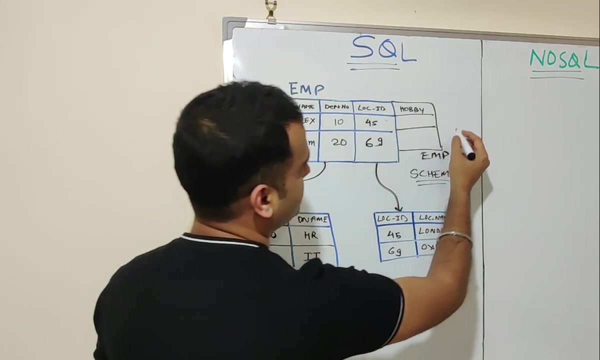 So it is kind of an optional field. It might not exist at all for that particular employee. So in this scenario we are seeing a change in the table format. We are having a new column being added here. It also can happen that you again have a request of taking the data of employees along with their contact information. 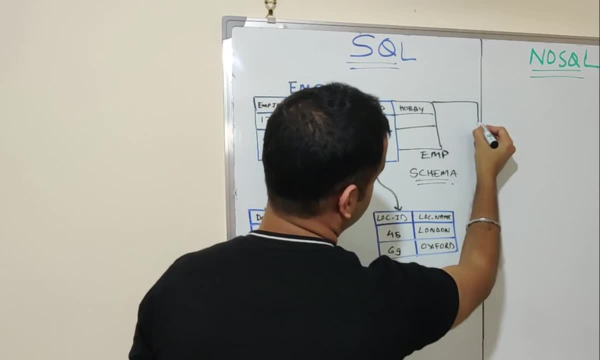 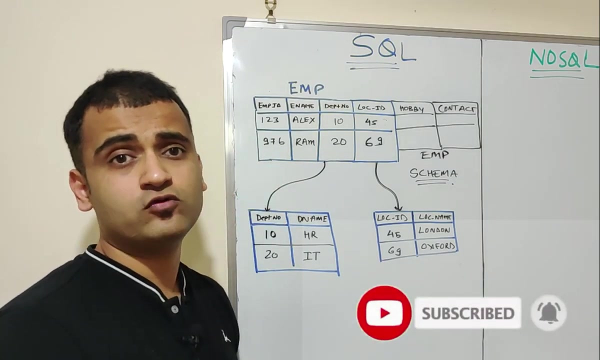 So there can be a change in the way data is coming And you can have another column like contact, where you will have the contact IDs of these employees, And one particular employee can have two telephone numbers: primary, secondary. The employee can also have primary and secondary email IDs. 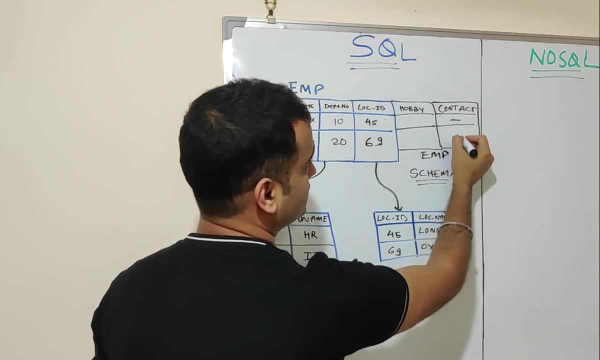 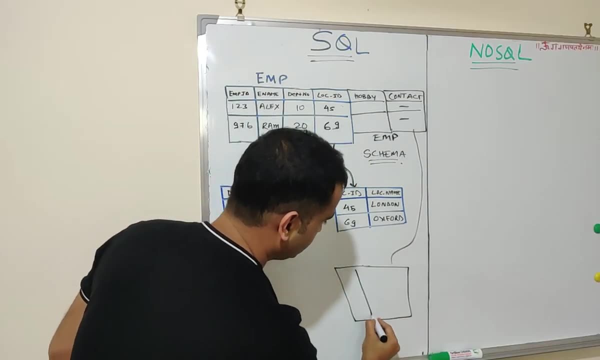 So basically you might want to populate some sort of a contact ID And then pretty much we are talking about a new table, And this particular new table will have your telephone number and your email And it might be having multiple records for one employee. 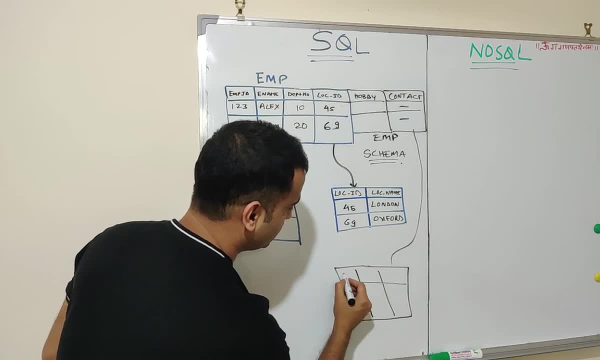 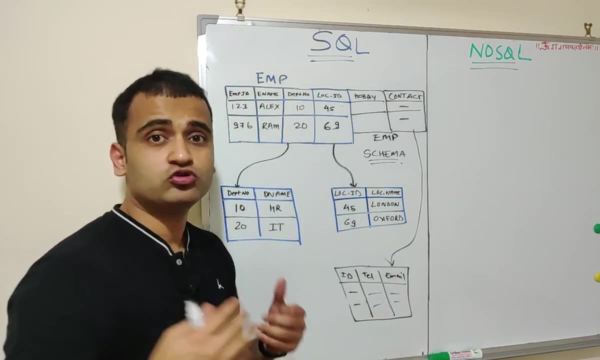 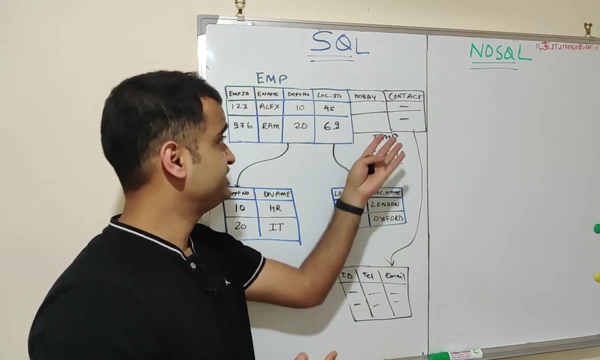 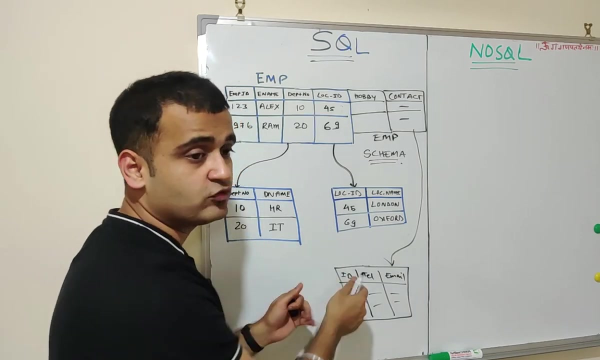 So you can- you know you can- have ID telephone email like that. OK, so just understand the kind of changes it requires for one particular change in the table format and how it gets populated into all the different tables you have to populate that. 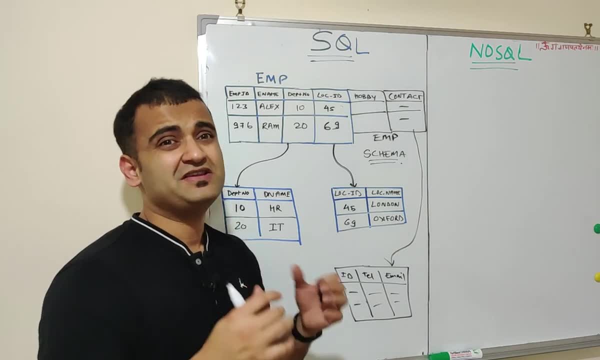 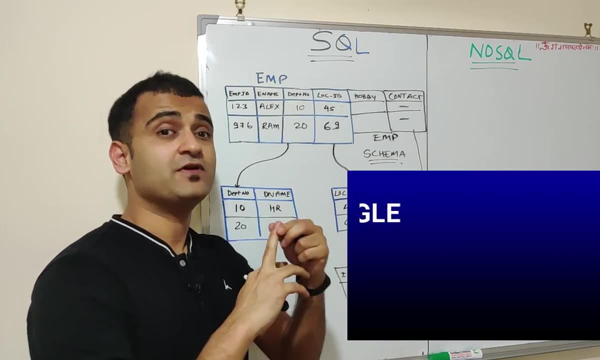 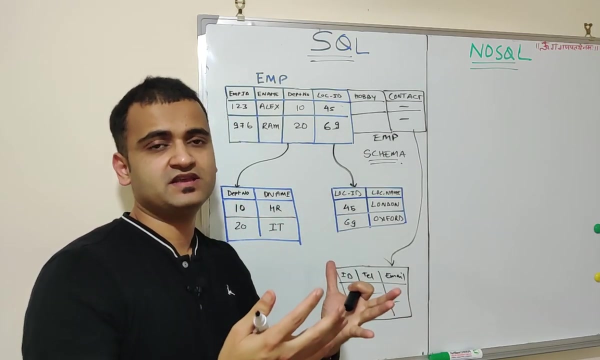 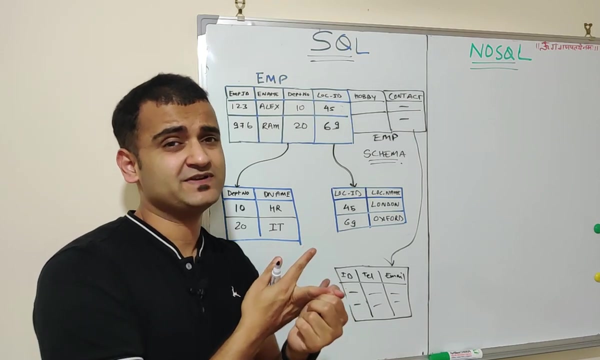 And that is where a traditional SQL database is not very flexible When it comes to high volume of data, high velocity of data and then different variety of data. OK, so whenever there is this kind of a scenario where you don't really know what kind of data to expect, you don't really know the pace at which the data would come. 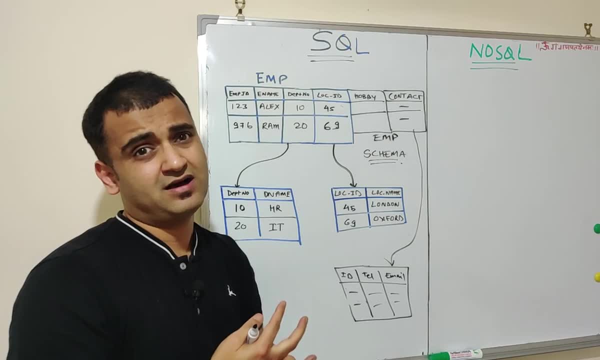 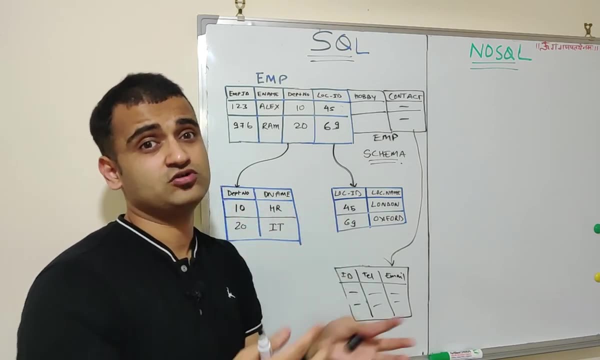 And you don't really know the kind of data which might come into your database, Then it is a perfect recipe to look for A new SQL database. And when I say that, by no means a traditional SQL database is losing its shine- It still captures more than 70 percent of overall market. 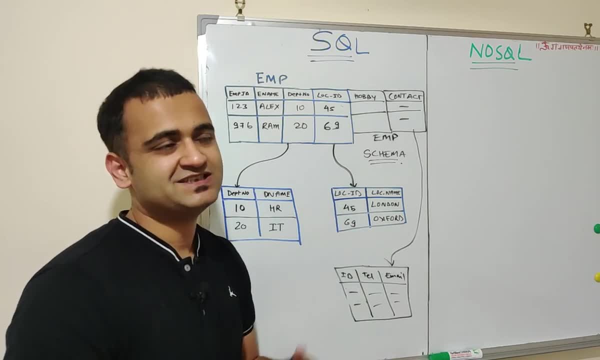 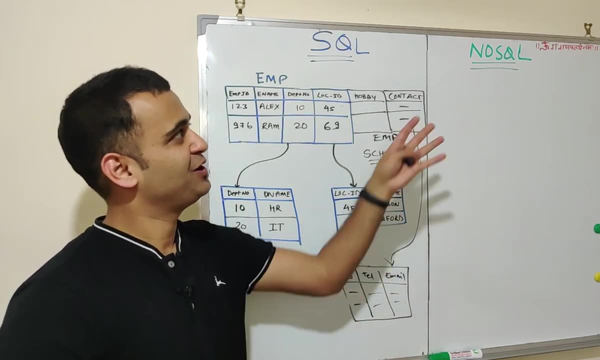 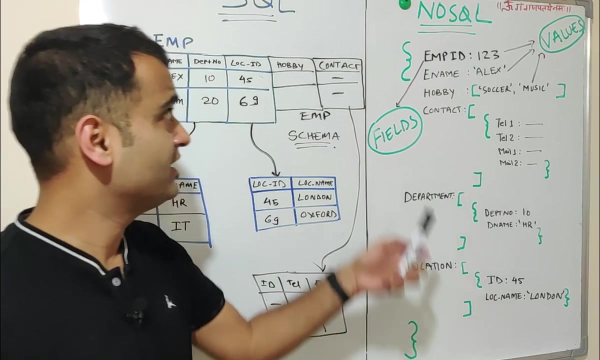 And with the new advent of technology, even a traditional SQL database can cater to a lot of scenarios. But let's now understand how a new SQL database would fit this particular employee data. OK, So, as you can see, we have encapsulated the whole employee schema into one document. 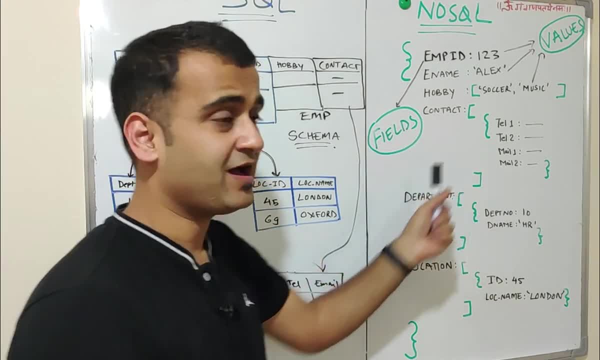 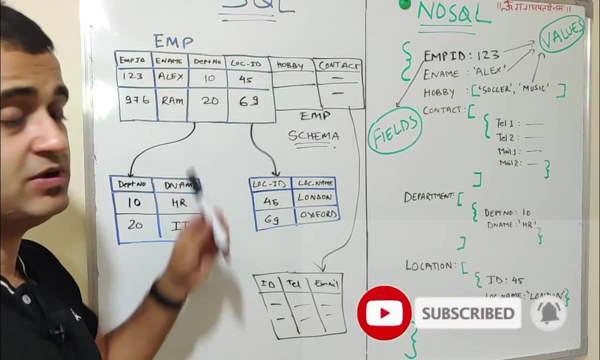 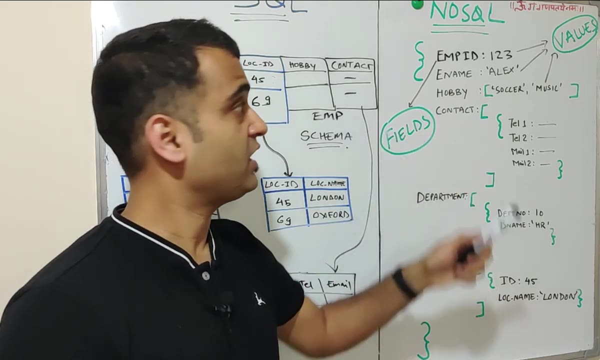 And pretty much whatever fields you see here are coming from all these multiple tables which were used And the data used to get stored in multiple tables. Now everything gets stored in one particular document, So in this case we are talking about data for employee Alex. 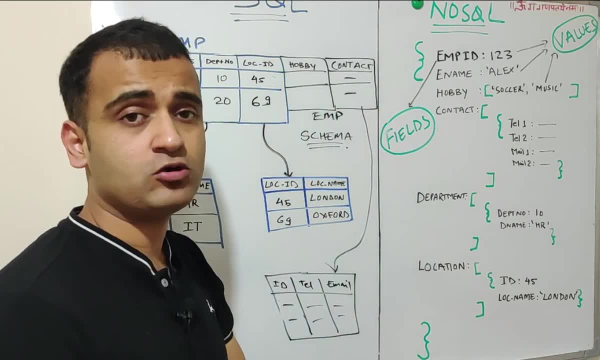 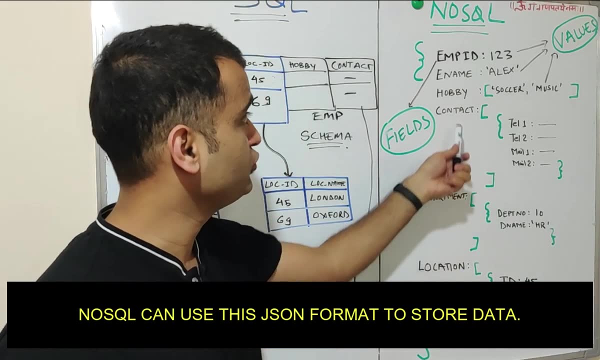 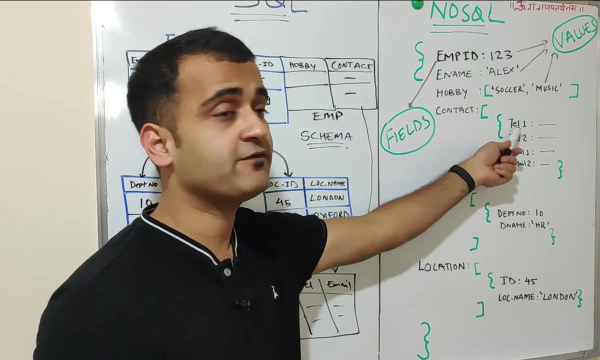 Every data which you see is now encapsulated in one document In the form of fields and values. You can have arrays of data within this document So you can have all your contacts within this particular array. So you might get a scenario where you are only having data for primary telephone number and primary mail ID. 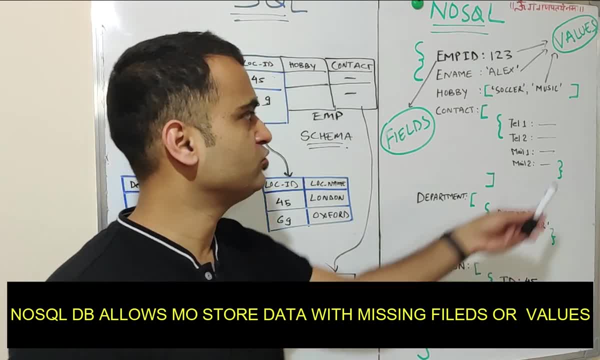 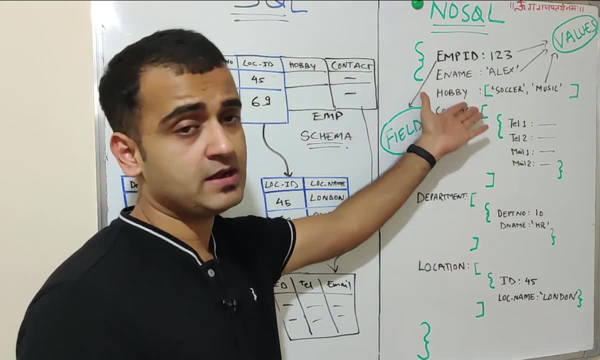 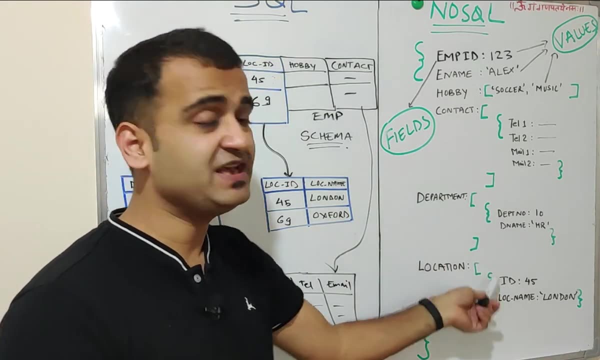 So it does not matter. in a NoSQL database, You can leave these fields empty. There can also be a scenario where you can get values for this particular employee, But you do not know against which field you have to tag that value. In that case, you can simply keep that value in the document and wait for that particular field to arrive. 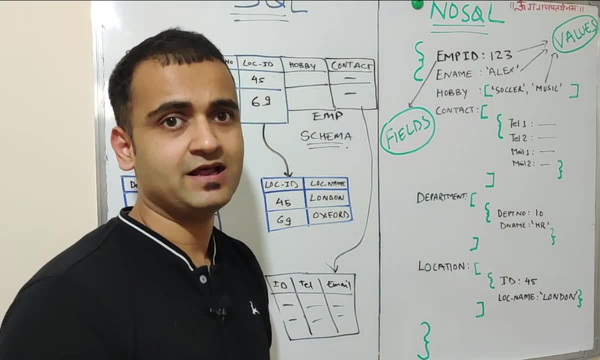 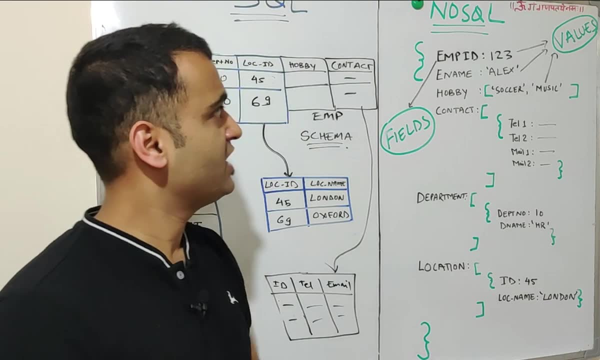 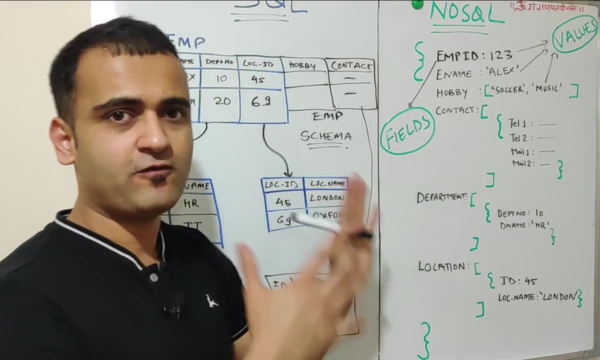 As and when it arrives, you can make this particular whole data set consistent, So you can understand how flexible it is to store data in such format. I have only shown this for Alex, But similar thing will follow for Ram as well. So this is a typical format in which you can store data into a NoSQL database. 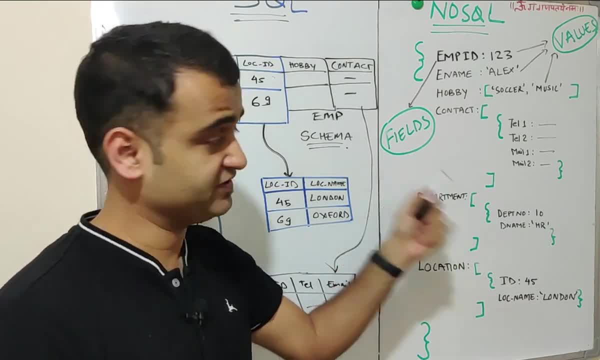 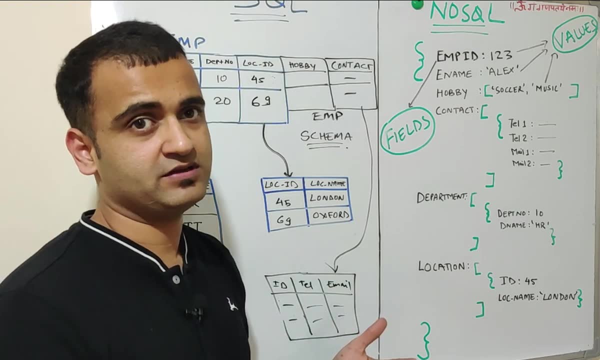 And this particular database is a document database, which I am discussing here, So you might have heard the name of MongoDB. It is a document database which is one of the type of NoSQL database, So in that the data gets stored in this manner, 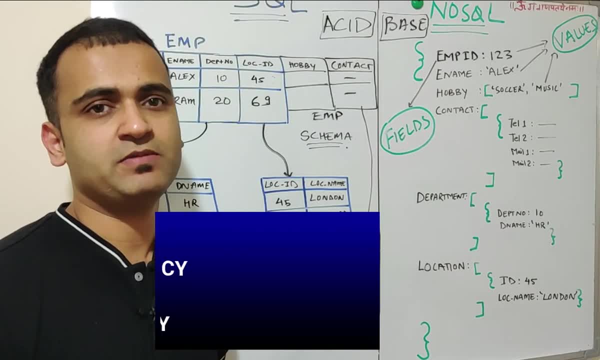 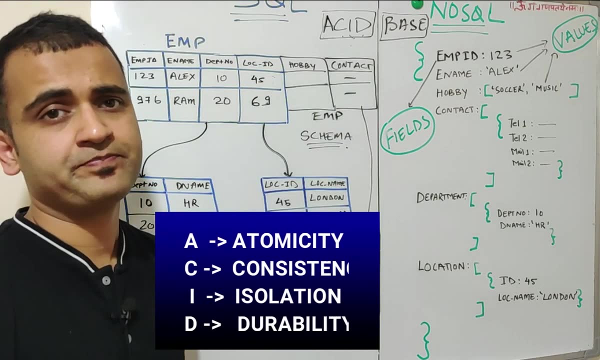 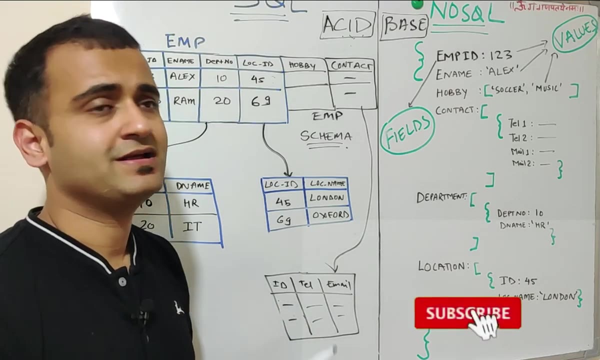 So all your traditional SQL relational databases follow ACID compliance, Which stands for Atomicity, Consistency, Isolation And Durability, And unless the data coming in matches this compliance, that data cannot be accepted in a relational database, SQL database. 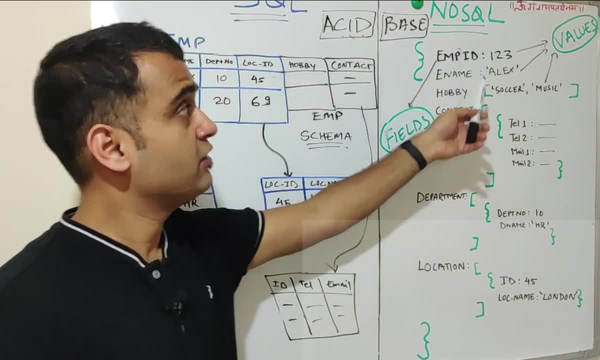 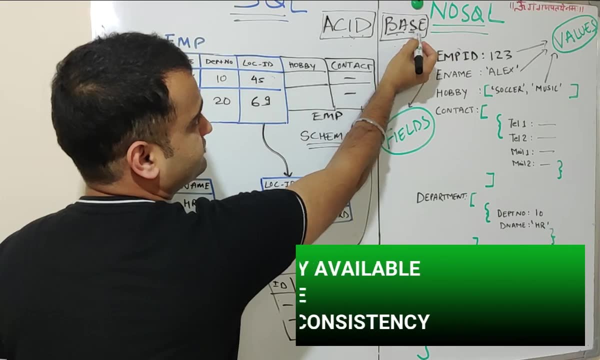 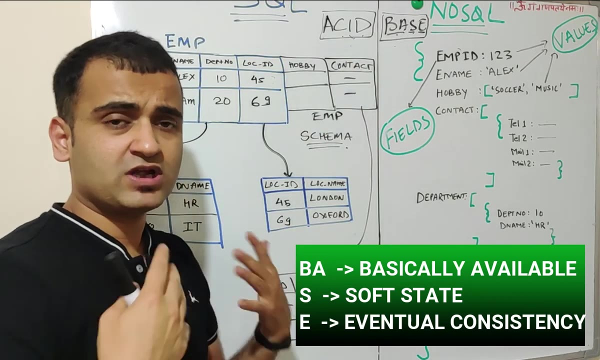 But on the flip side, a NoSQL database follows BASE principle. So BASE stands for Basically Available, Soft State and Eventual Consistency. Now let us understand that Basically Available means that pretty much whatever data which tries to come into a NoSQL database would be available. 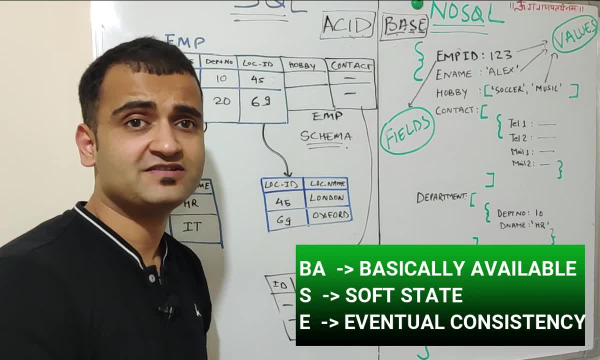 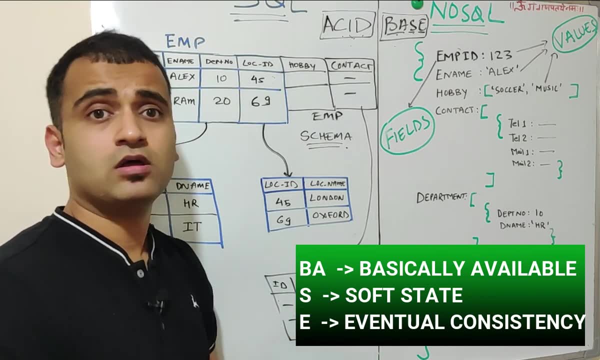 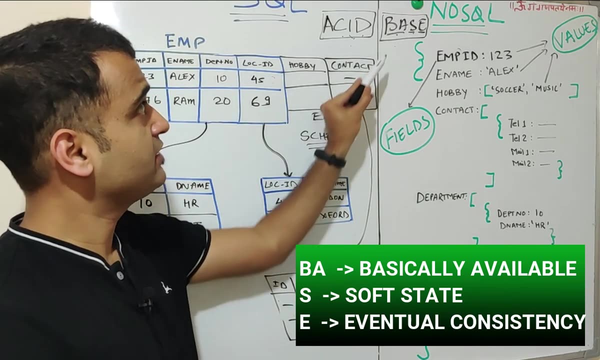 There might be scenarios where you might encounter failure state Because the data which is coming in might fail to enter into the system. Overall, the data would be available in the database sooner or later, So this is called as Basically Available Soft State. 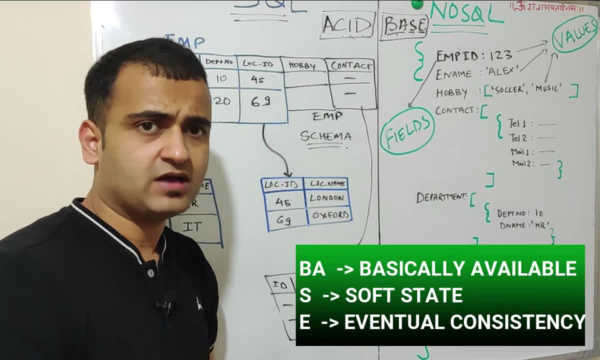 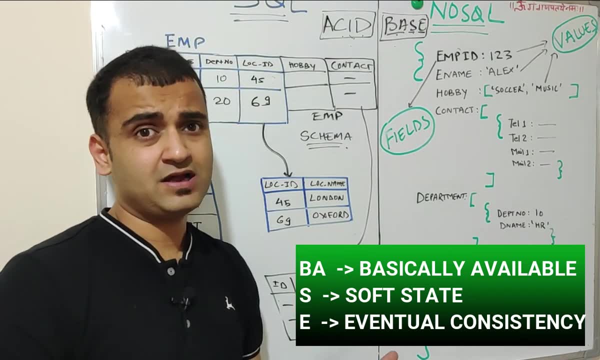 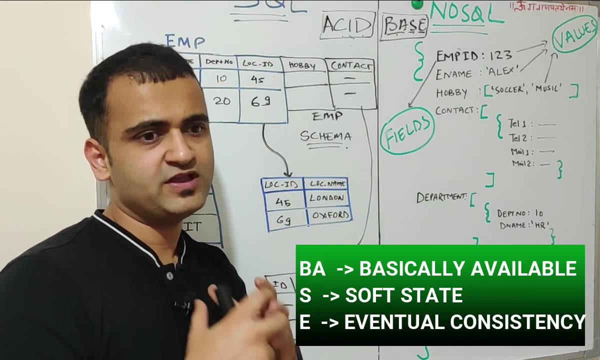 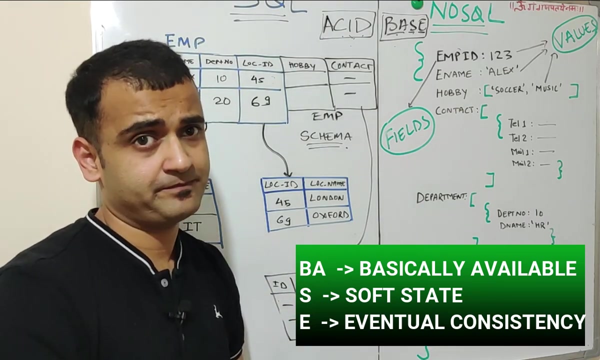 Soft State means that the data would continue to vary over the period of time. Because of its flexible database design, you might encounter that you might see changes very frequently in your data, which is coming, So there will always be a Soft State. That Soft State means that the data could vary over the period of time very frequently. 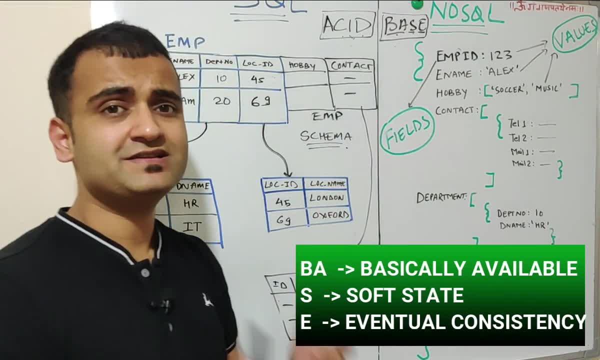 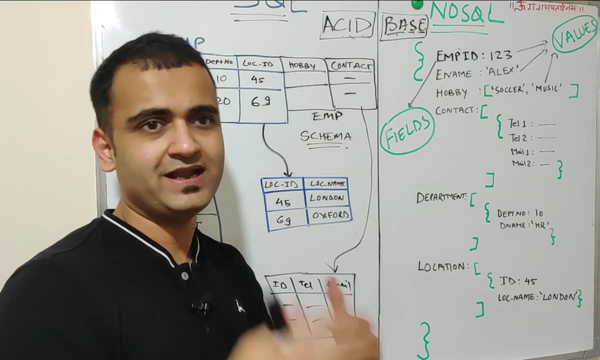 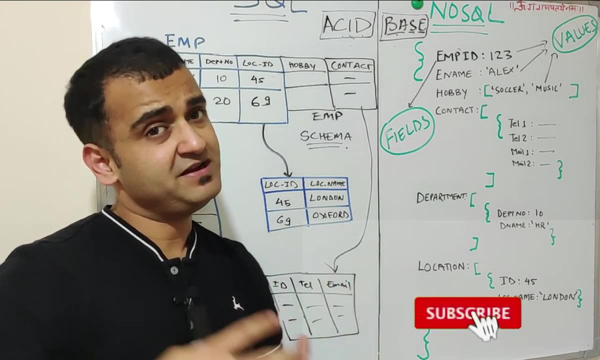 Eventual Consistency. Eventual Consistency means that regardless of what kind of data is coming in, it might not be consistent while it is being fed into the database and getting stored in whichever format possible, But eventually, while reading the data, when all the data inserts and the data loads are finished, 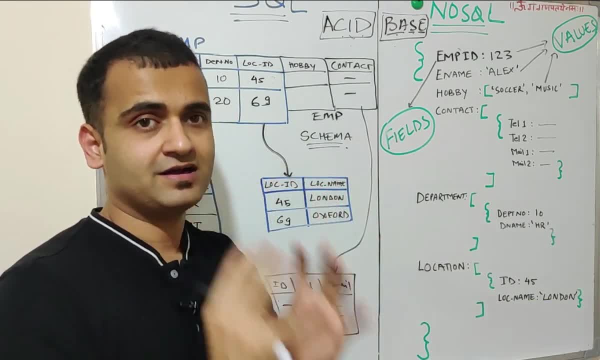 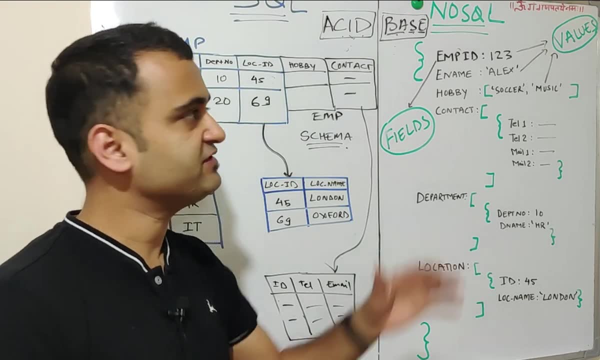 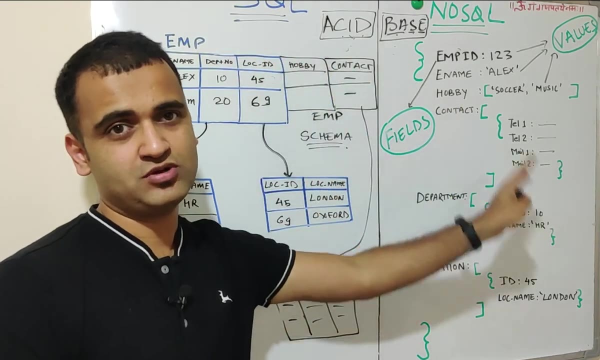 the system will eventually make all the data consistent. So that is a very, very important difference between a traditional SQL database and a NoSQL database. So this is a basic understanding of what is SQL versus NoSQL database. I think you have now got an idea. 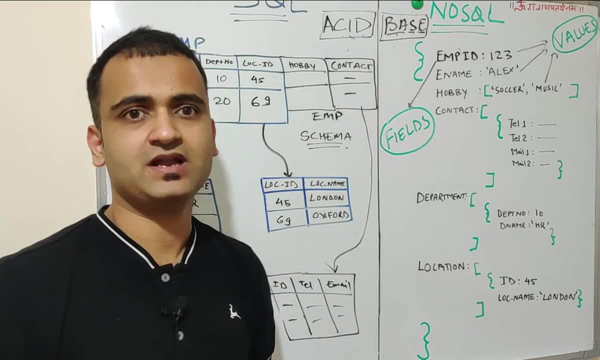 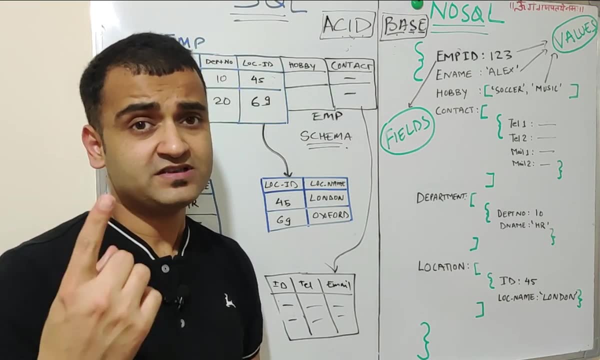 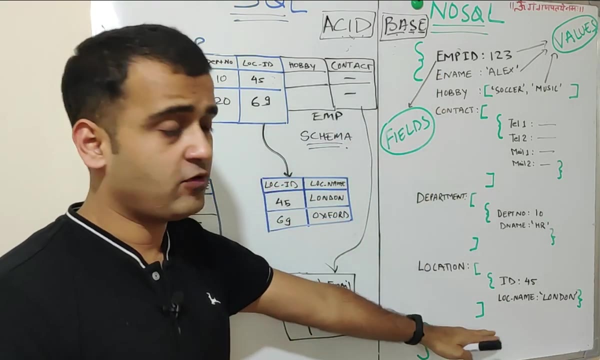 Now quickly understand what kind of NoSQL database we have in the market. So if you have to categorize, you can categorize it into four different categories. First, you have already seen it is a document database. As the name suggests, the data is stored in the form of a document. 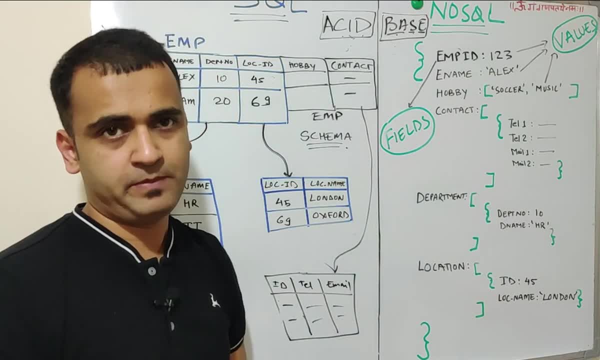 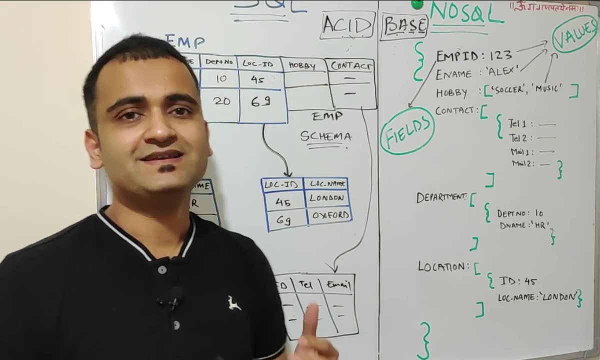 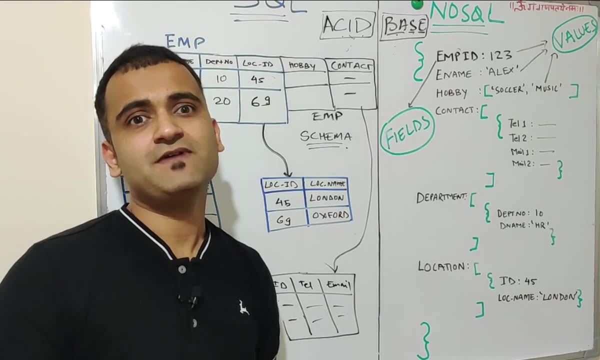 And in the form of fields and value pairs. Famous example: MongoDB. MongoDB is a famous document database And this is currently used in companies like Uber. Second type of database is a key value pair database. What is a key value pair database? 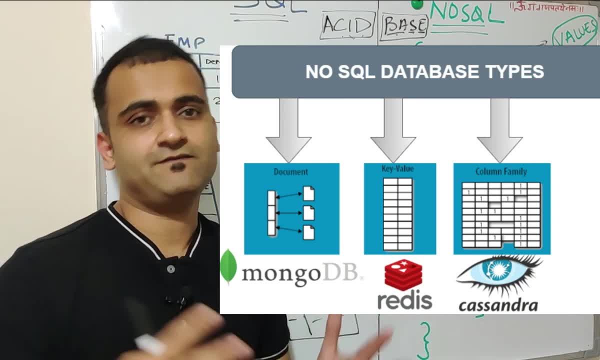 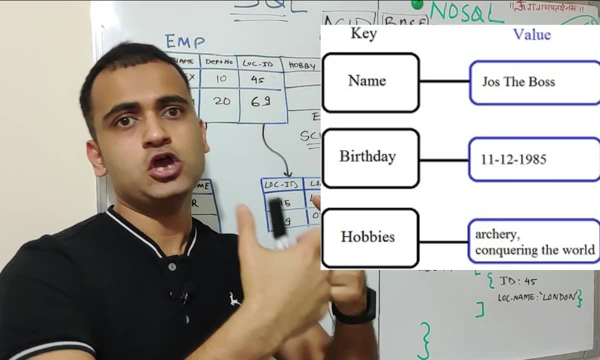 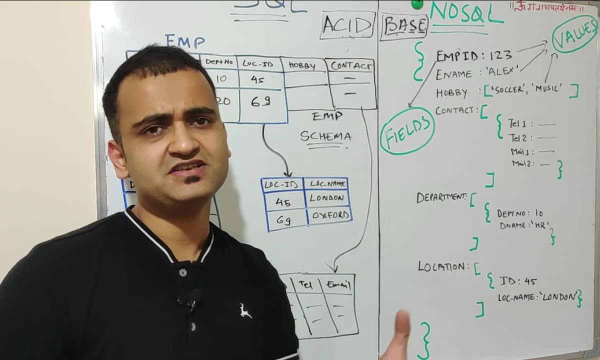 So it works in the form of key and values. You will have a hash key And in correspondence to that hash key you will have a value associated with that. So you can take an example of a dictionary. In a dictionary you search for a word and then you get the meaning of that word. 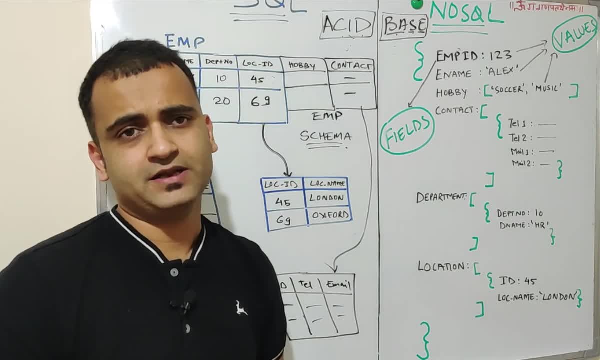 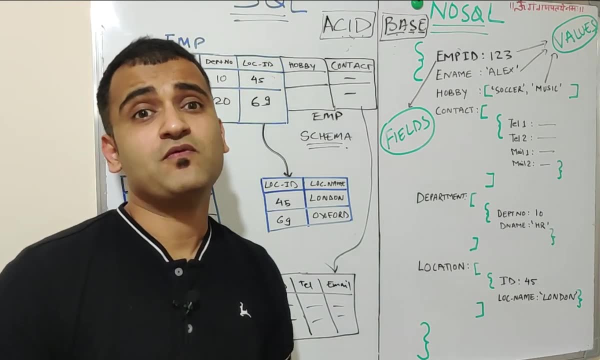 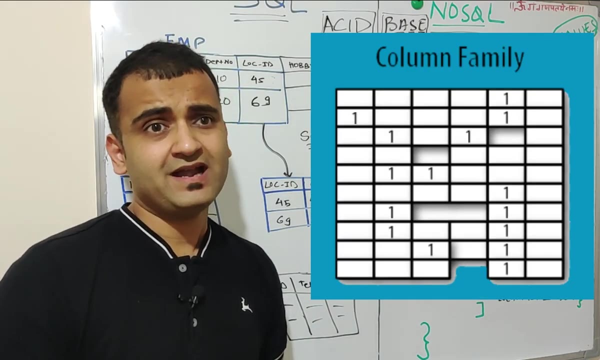 when you search through that particular word in the dictionary, The famous company using key value is Twitter and Pinterest. Third type of database is wide column database. Now, what is a wide column database? A wide column database works on the phenomena that you can have an equal number of columns for each specific row. 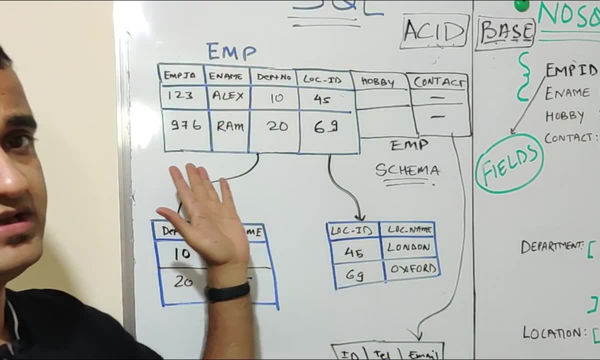 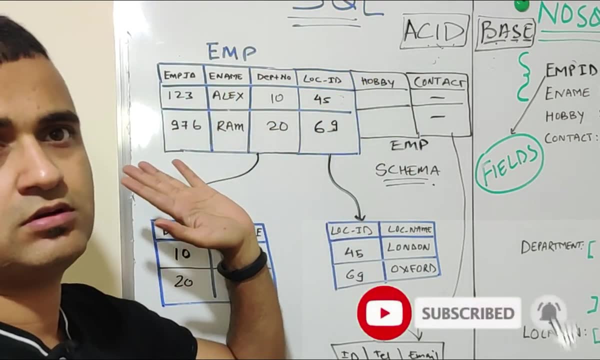 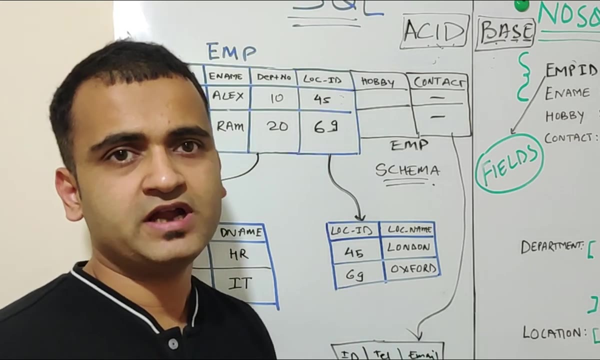 So suppose you have this employee table And in this employee table you have one column which is only specific to employee Alex Rest. all the employees does not need that particular column. So in that case a wide column database because it stores the data. 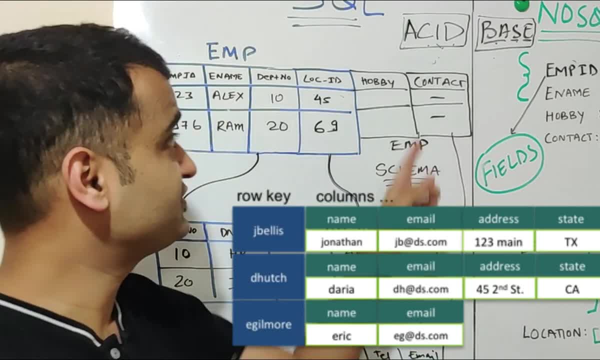 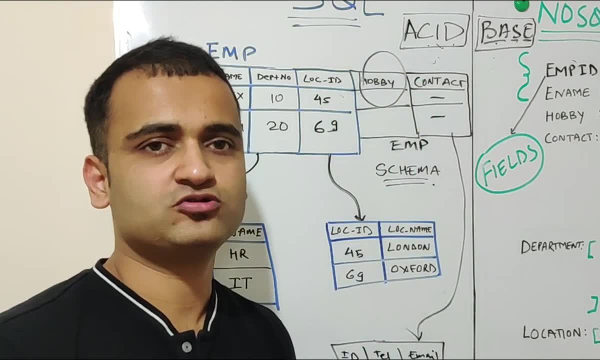 based on specific columns, so it will ensure that it stores the data only for this particular row and this particular column. So this is also a famous type of NoSQL database: wide column database. Cassandra is a very famous product for wide column database. 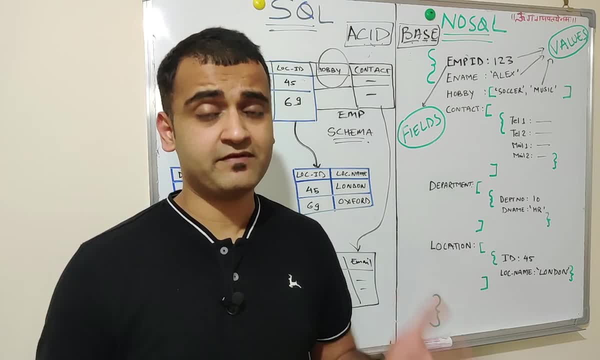 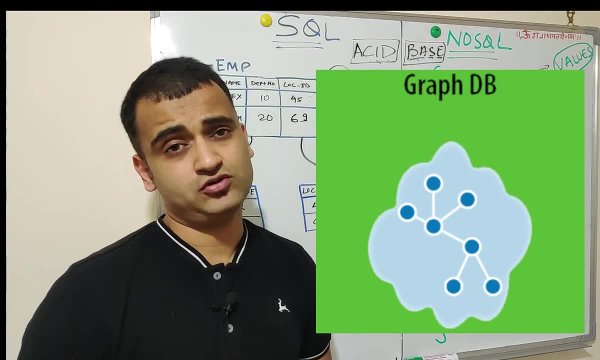 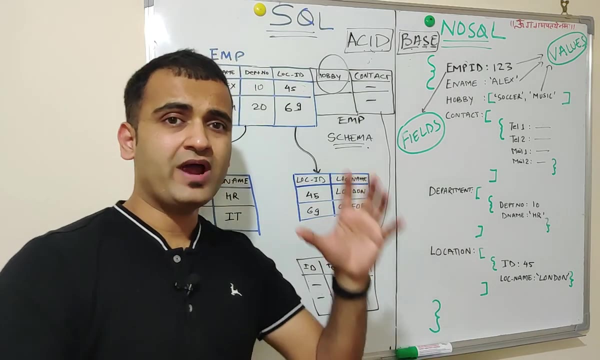 So famous company using wide column database, that is, a Cassandra database, is Netflix. Last type of NoSQL database, that is GraphSQL. Now, as the name suggests, what is a GraphSQL? GraphSQL divides your data into entities and the relationship between those entities. 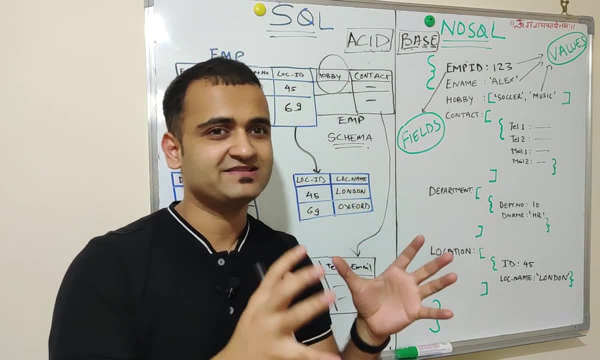 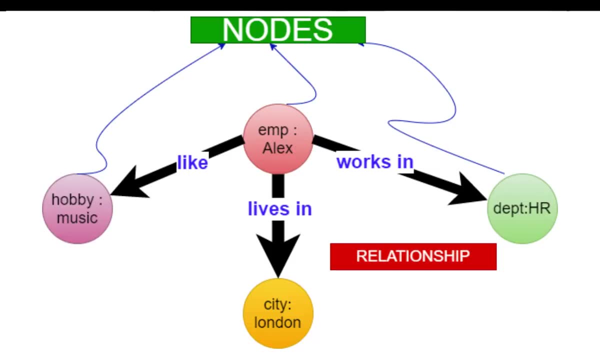 You might correlated with an entity relationship diagram, but not exactly. Basically divides your entities into nodes And those nodes connects to a different node through a relation And in case of employee table you can have employee as one entity, one node And that particular node. 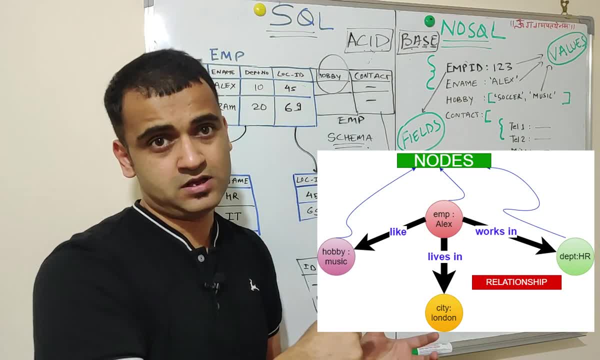 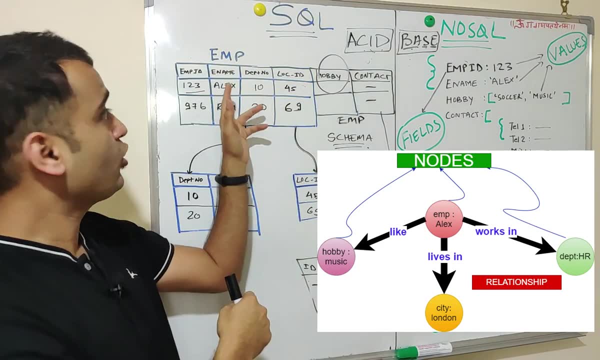 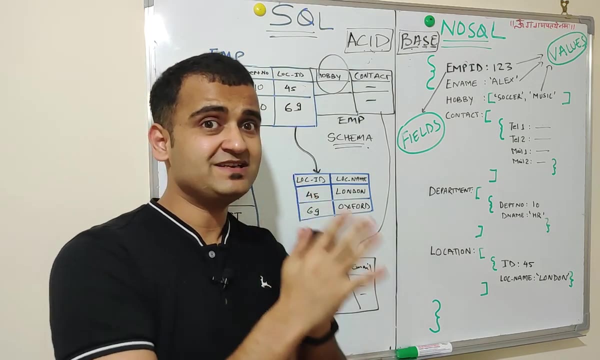 connects to a department node And the relationship between employee and department would be working in, Working in would be the relation Employee Alex is working in HR department. But the difference is that, because you have explicitly defined these relationships, these relationships remain static. 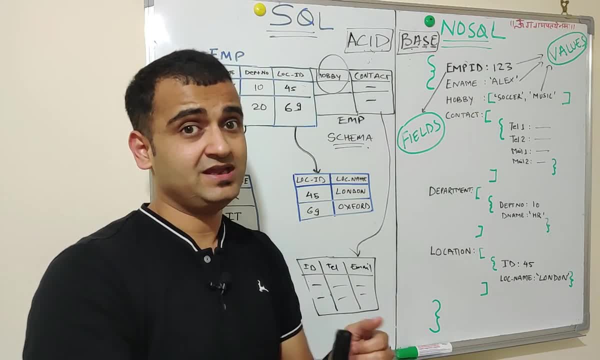 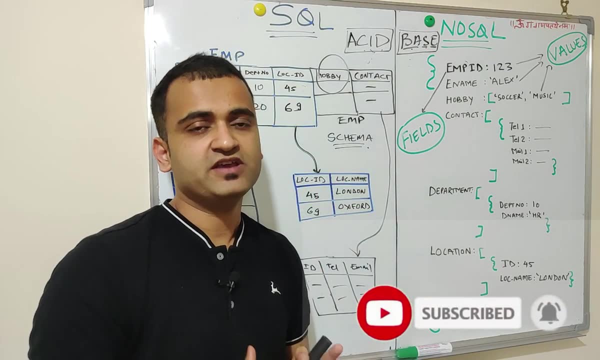 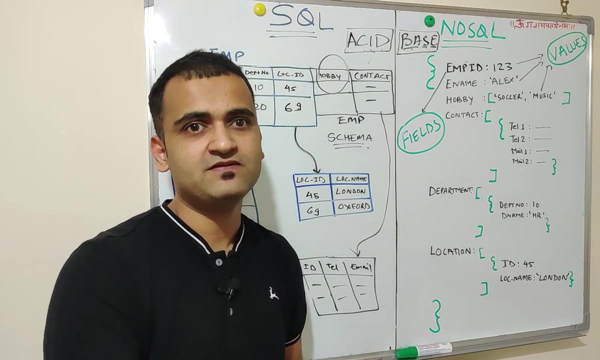 What does that mean? That when you run the query on a GraphSQL database, the outcome is very fast Because all the relationships which you make in a Graph database are very, very clear, predefined and there are no changes Once a relationship has been formed. 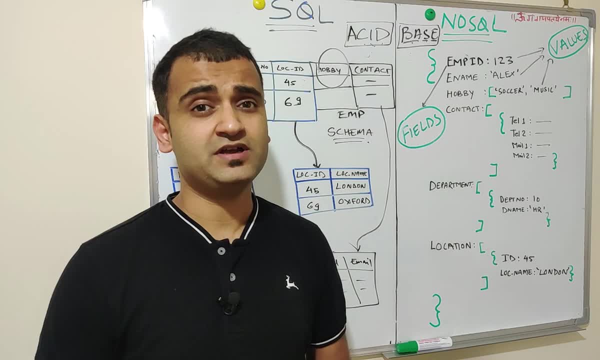 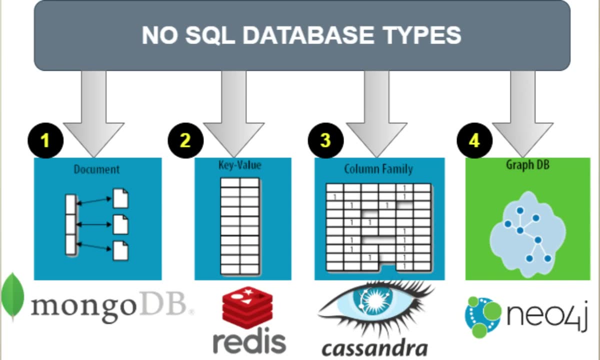 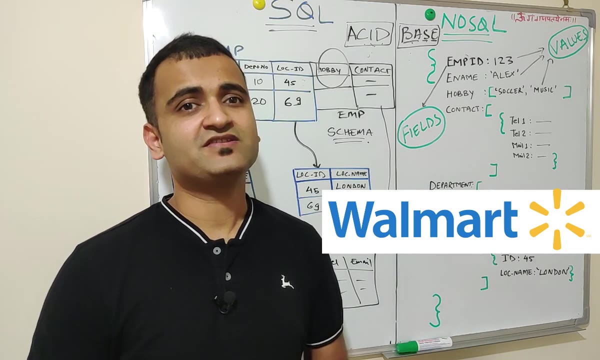 it can not be changed In case of GraphSQL database. Neo4j is a famous product which is used widely by various companies. One very famous company using GraphSQL database via Neo4j is Walmart. So, friends, just to recap,